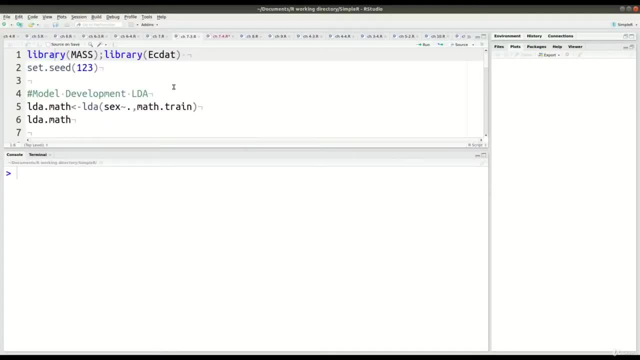 having said that, let's go ahead and go over to R. So first you have to run your libraries in line 1, set the seed in line 2, and then, in lines 5 and 6, we're going to run our model. 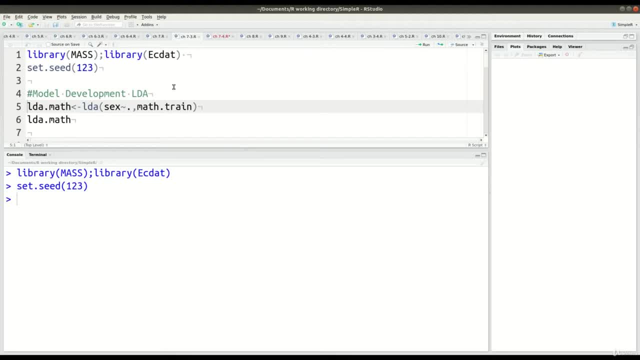 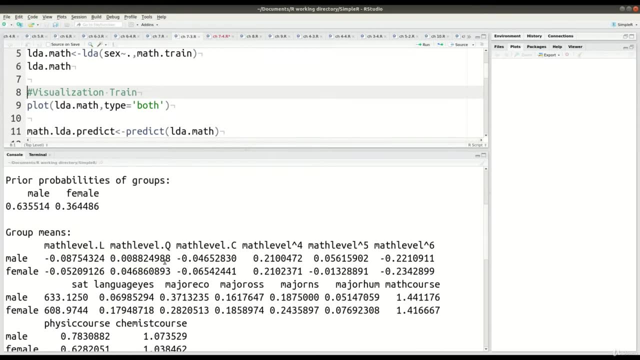 using linear discriminant analysis. So I've explained that. I've explained this before, so I'm just going to do it quickly here. So here are the results right here for our data. and so all this information here is the means for men and women for the 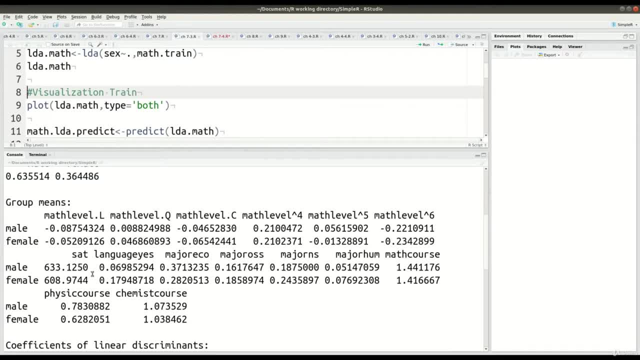 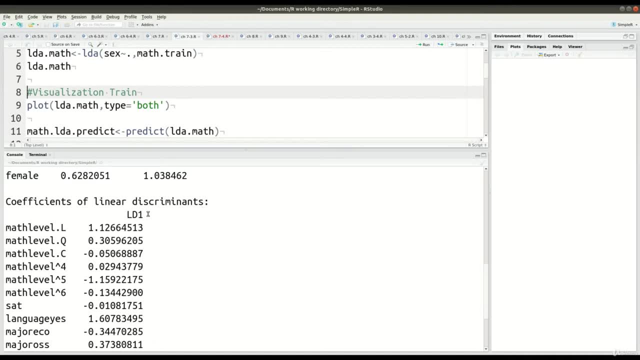 different variables. Now we use these means, we use these differences here to try to set up our linear discriminant function and then down here below we have the coefficients. Notice how we only have one linear discriminant. That's because the number of lines of discriminants 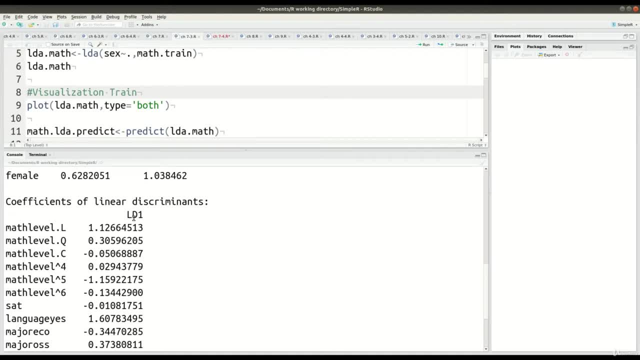 are made based on the number of groups minus 1. Two groups, men and women, so that's 2.. 2 minus 1 becomes 1.. That's why we only have one discriminant analysis here, So you can see the different levels etc. Now having 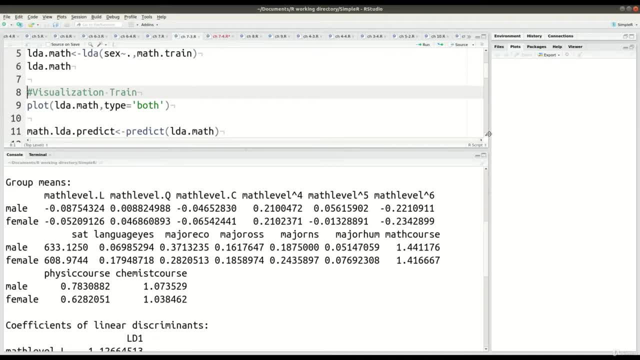 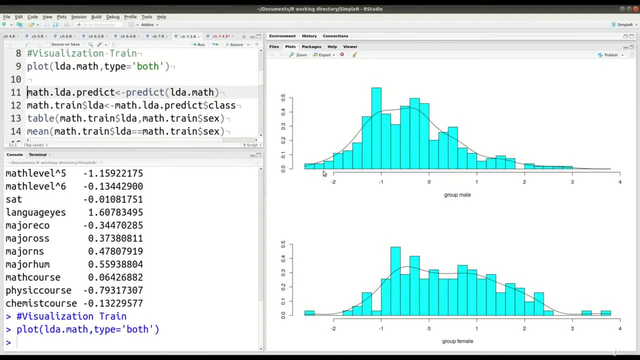 said that why don't we take a look at the visuals? This will be a little bit easier for us to try to understand what's happening with the data, so I'm going to make that bigger. And then, in line 9, we do our first visual, And so here's kind of the distribution for 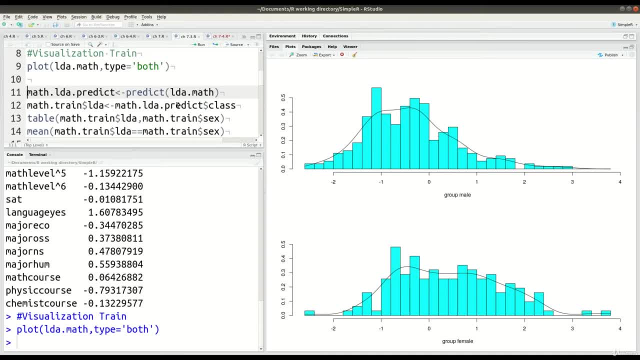 the males and the females. You can see that there's a little bit of overlap, which means we might have some challenges in terms of our predictions here. Now, in line 9, we have a little bit of overlap, which means we might have some challenges in terms of our predictions here. 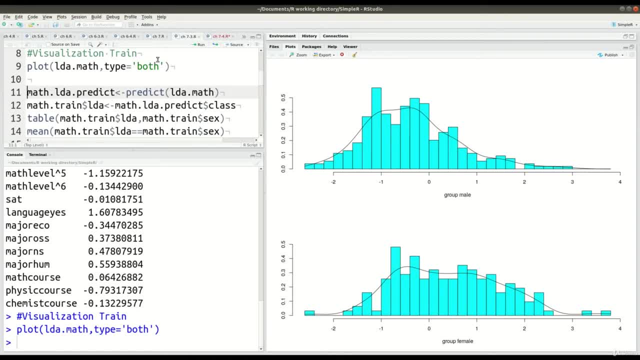 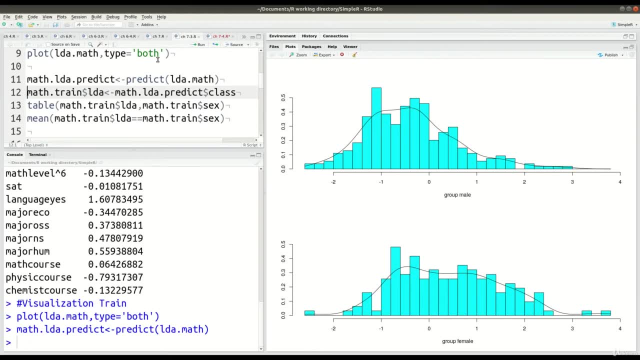 Now in line 9, we do our first visual, And so here's kind of the distribution for the. now in lines 11 and 12 we start to. in line 11, excuse me, we do our predictions um based on our data, and then in line 12 we we um pull the, the predictions that come from the math ldapredict. 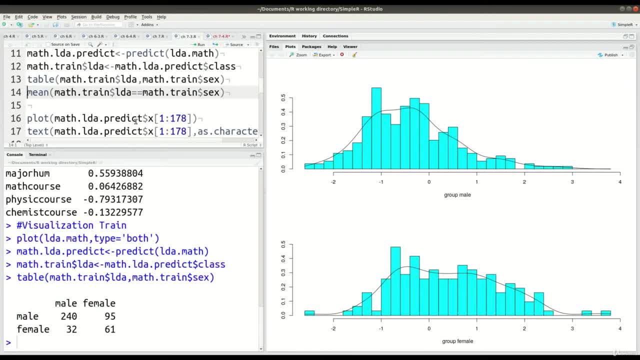 and then the lines 13 to 14. we make our table and get our our um, what do you call it? our accuracy rate. so you can see here, down here in the corner of the accuracy here, uh, so 240 out of the males were classified correctly, 6100 females were classified collecting. we have some problem. 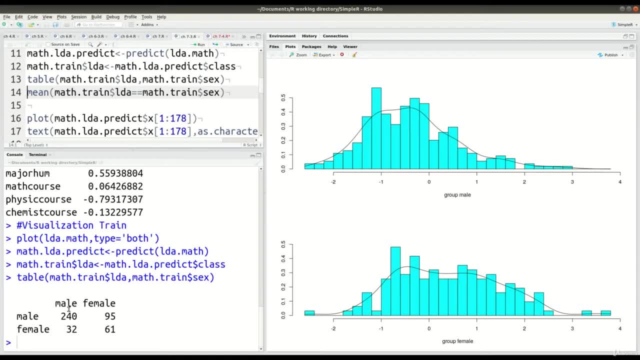 with some males being judged as females and of course some females being judged as males, etc. and then for our accuracy we use the mean function and we do math dot train dot uh, dollar sign lda. and then we do math dot train that sex lda is like the prediction. that's what i called it. if 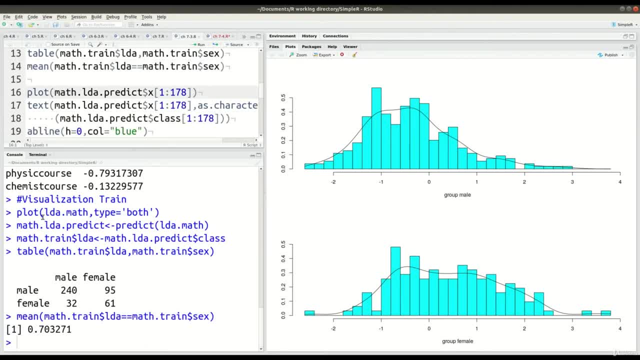 you look here in line 12 if you will. so we do that and you can see we got about 70 accuracy. that sounds pretty good, and so now we're going to make a picture of the actual distribution. now this is the training set, and so obviously you know we can't put everything in the training set. 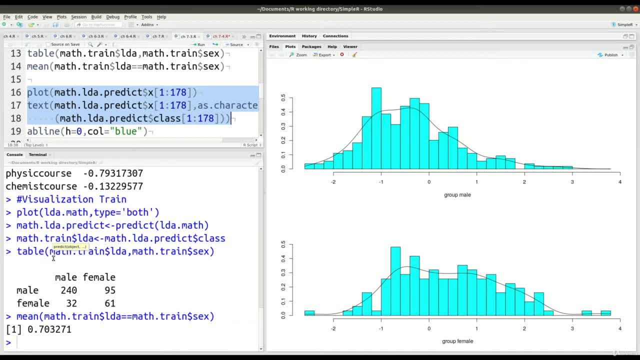 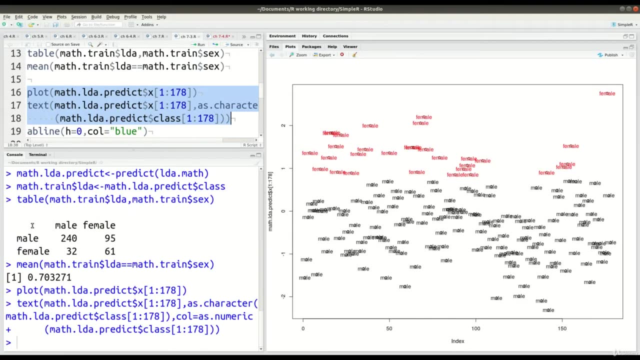 because we'll get a giant blob of black mass. but i chose 178 as our, as our example, because that's how many are in the test set. so it's good for for um comparison. what i mean by 178 is that we're taking the first 178 rows and we're going to map them on a plot, see what they look like, and so there. 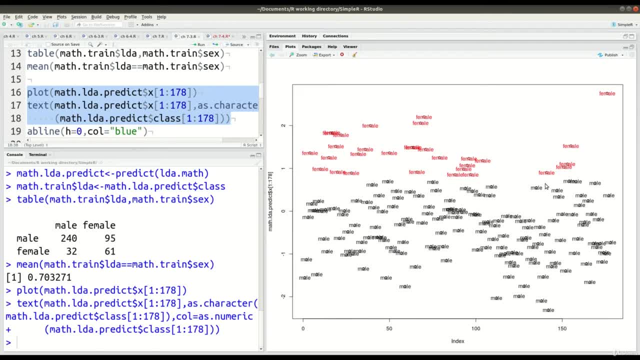 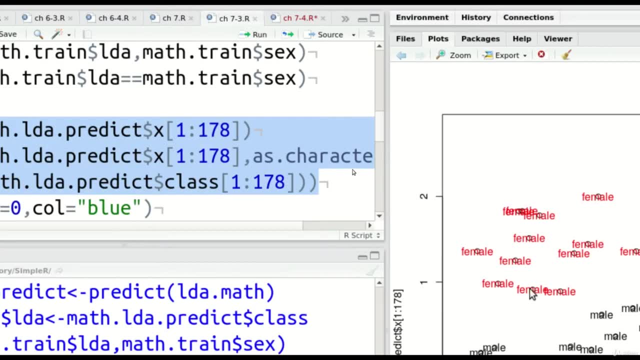 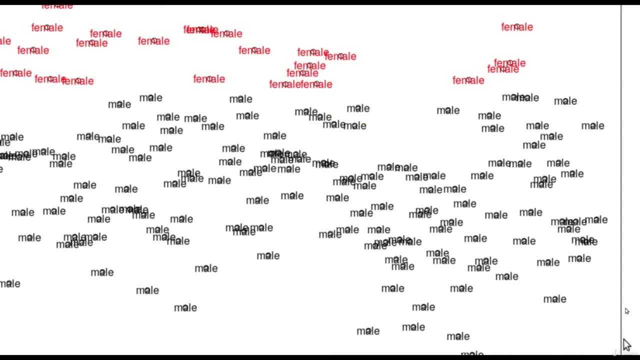 you can see they're clearly right there. there's a pretty good uh definition here between the males. let me zoom in for you so you can see this a little bit better. it's like, so you can see, right here the blacks are the males, the um the red is the females, and so it looks like it's a pretty 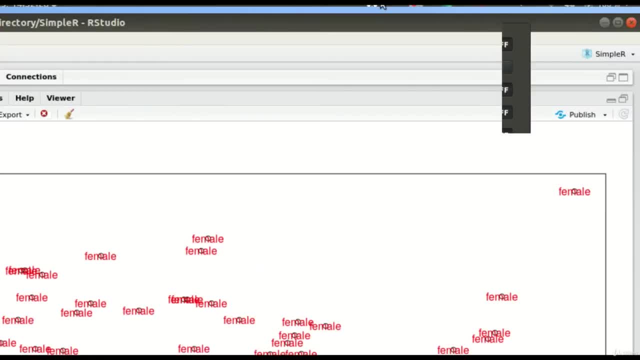 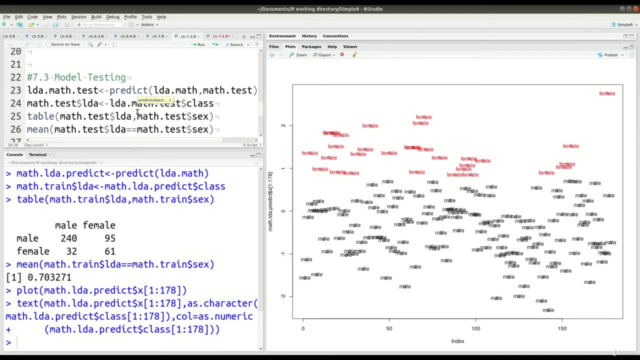 good. separation- 70, depending on what your goal is- could be pretty pretty uh good in the social sciences. we would normally be happy with that. so that's our uh, that's kind of what's happening with um, the visualization of this for the training set now for the test, or actually, i guess you can say: 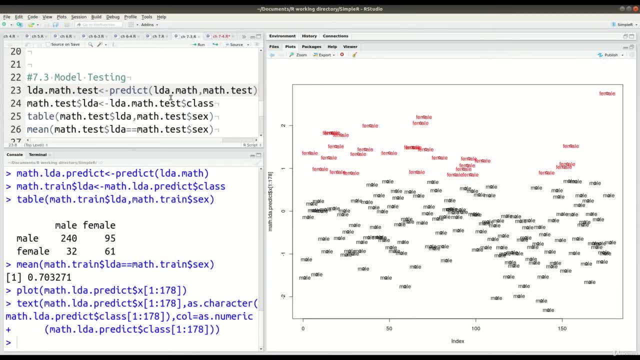 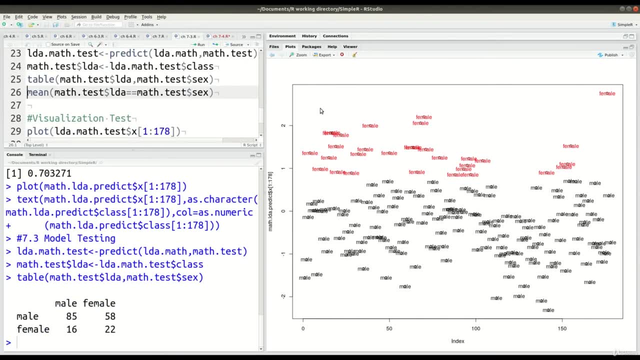 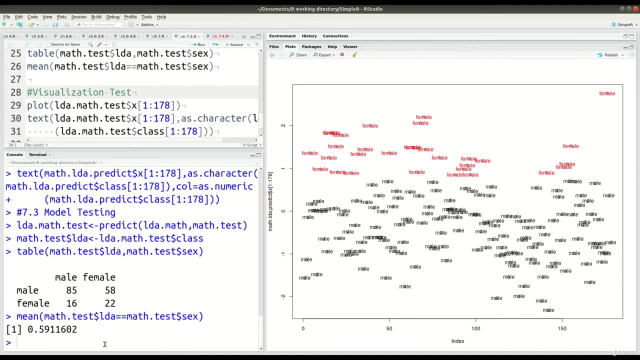 we take um our model. we made ldamath and we use now the test set, mathtest, and we run our results here again. this is most review, nothing new here. and you can see right here: uh, what's the accuracy in line 26: 59. so there's quite a bit of a drop off. this means that we're we're having a difficulty um. 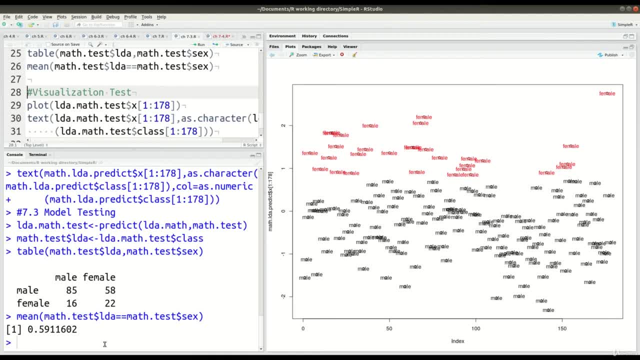 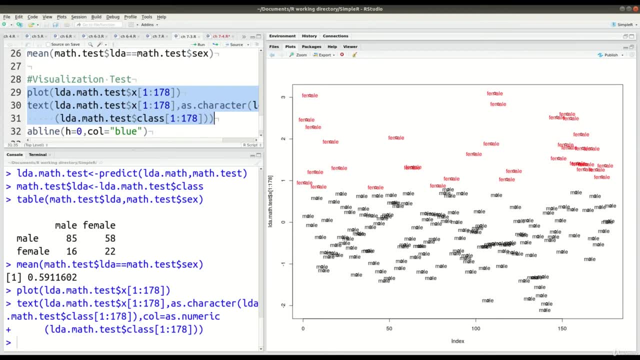 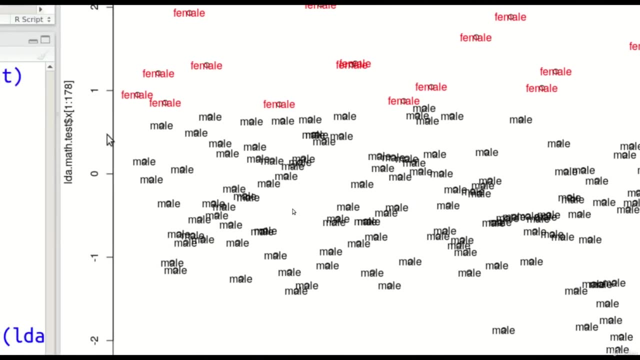 uh, using our model in a different context, it's not generalizing. well, and then for the visualization, we'll just run this so you can see here the spread of the data again. i'll zoom in just so you can look at this again. it looks like good separation, but we're not quite sure where the line is being drawn at. 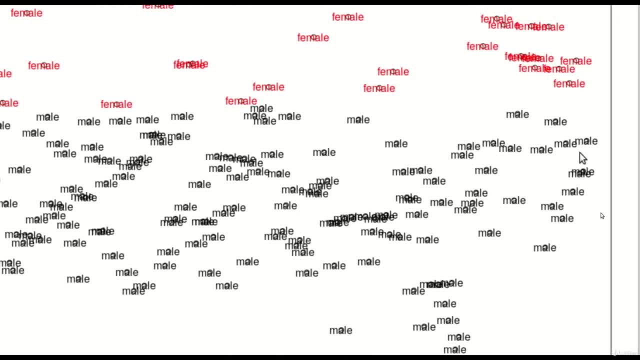 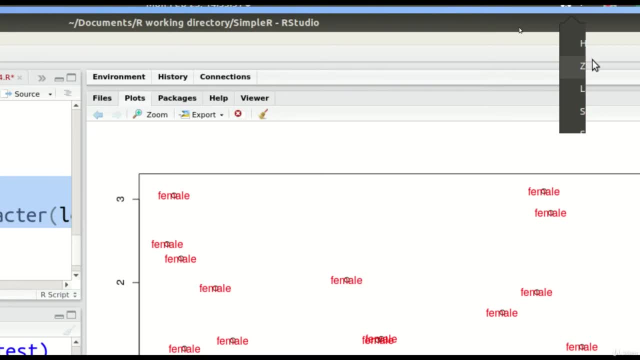 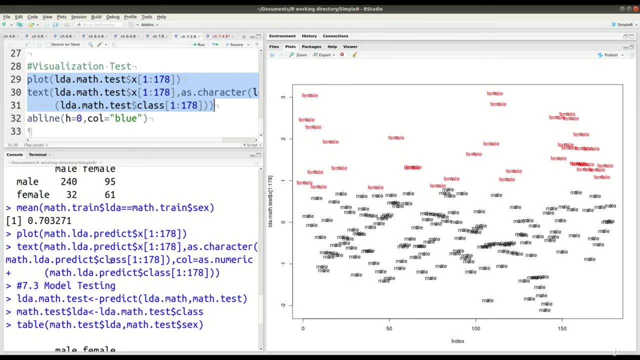 often it's drawn at zero- not always- and so that might be why. but remember, we don't have all the data here, just the first 178 rows, so it won't be completely clear, but we do have some idea of what to expect. all right, and so that pretty much wraps up this video, the key thing to remember as we walk. 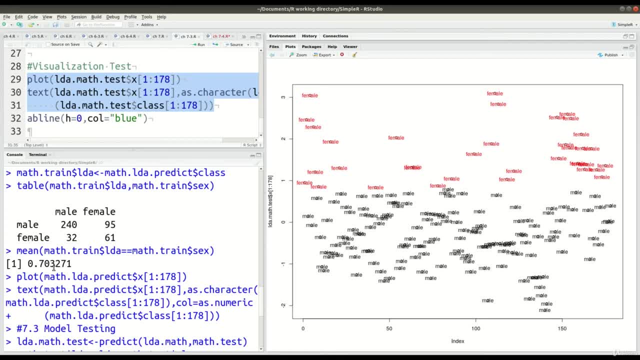 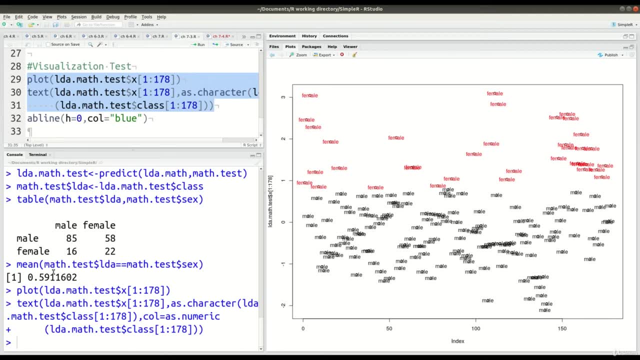 away from here is the accuracy of the data. so we're going to go ahead and zoom in a little bit and look at our analysis here and we're going to see how, what we did with our analysis on the table, did we reach for accuracy? so, on the training set, it was 70. on the test set, it was 59, and so now. 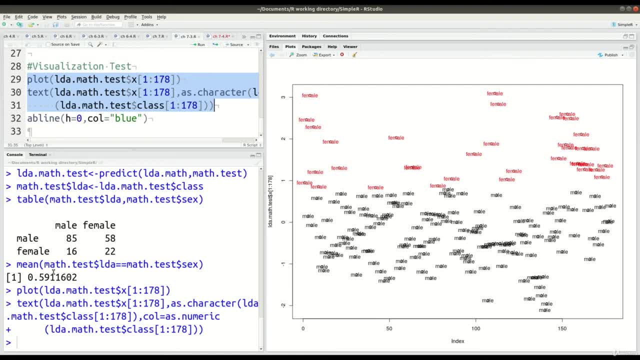 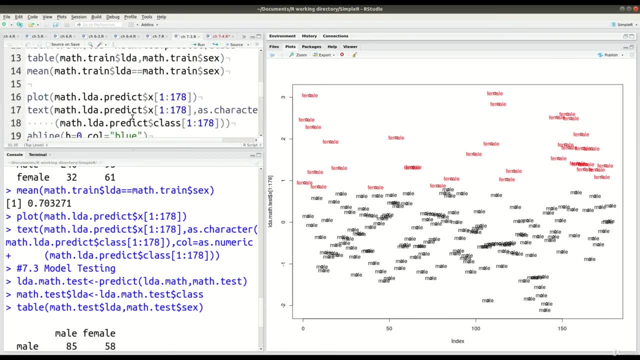 in the next video we're going to see, when we do this with quadratic discriminant analysis, how it will compare to what we did with linear discriminant analysis. so in this video we just ran a linear discriminant analysis model. this is a review of what we did in chapter 6. there's nothing. 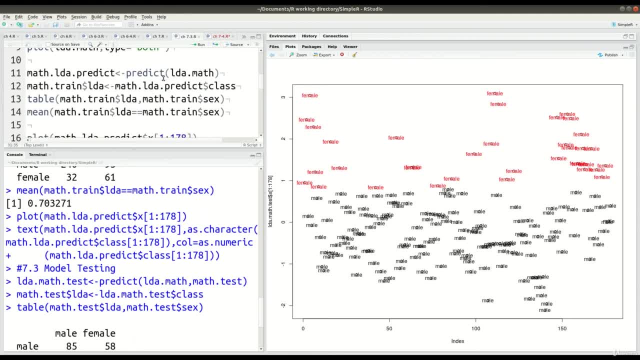 really new or radical here in, in particular: um, we, we did the plot, we ran the model. uh, we had a lot of do, a little bit of making a classification, where we had to take some information from different places. but again, this is almost a review and so i'm not going to spend a lot of time talking. 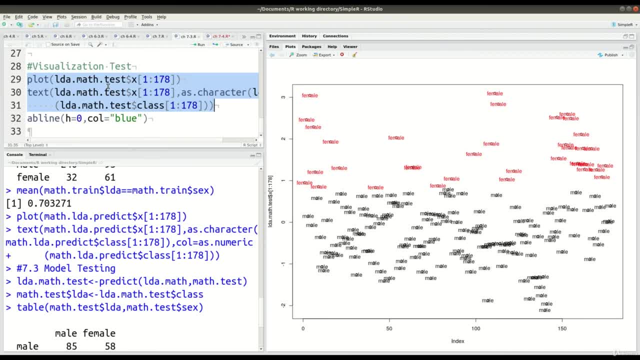 about this, so i hope this information was useful for you and i'm looking forward to seeing you in the next video when we do this, all this again with quadratic discriminant analysis. so my name is darren thomas. i am the director of educational research techniques. this is simpler using machine. 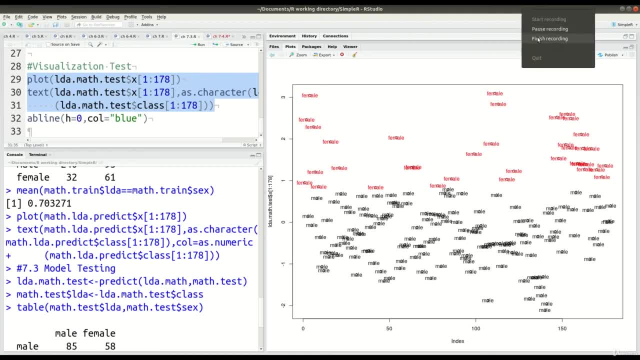 learning algorithms in r take care. 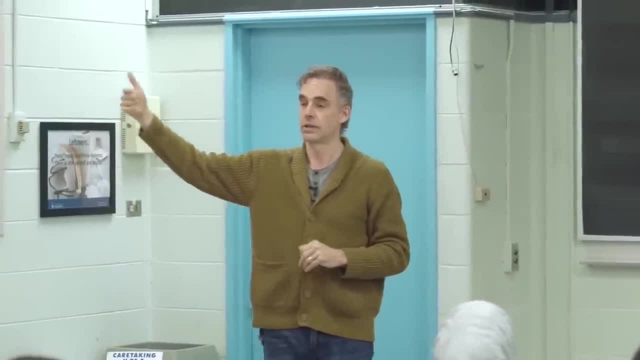 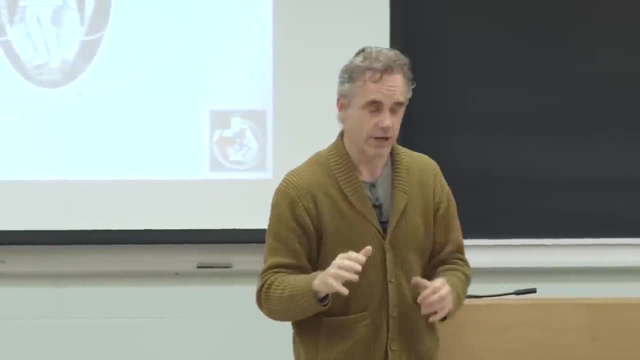 Men use the image of female perfection to motivate themselves, and that's exactly right. That's precisely what they do. You see that in the Tom Sawyer story. So Tom Sawyer is about 12 years old and he's still hanging around with his friends, like Huck Finn.